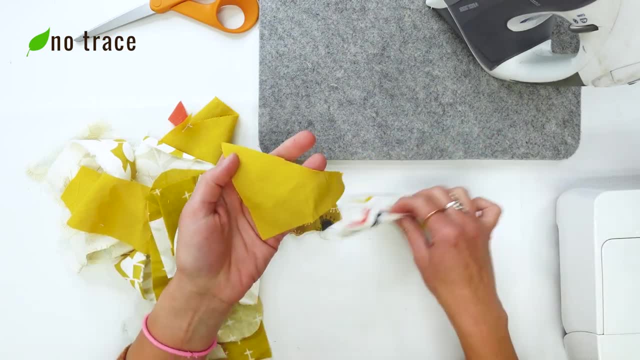 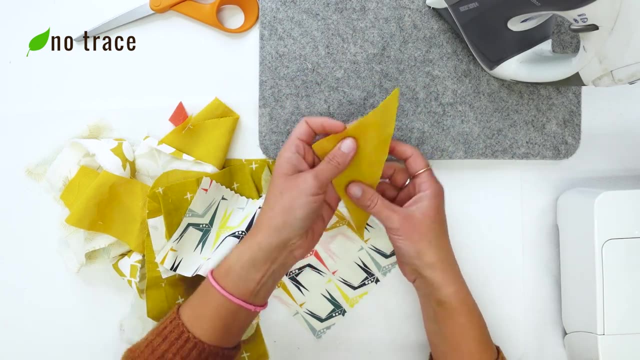 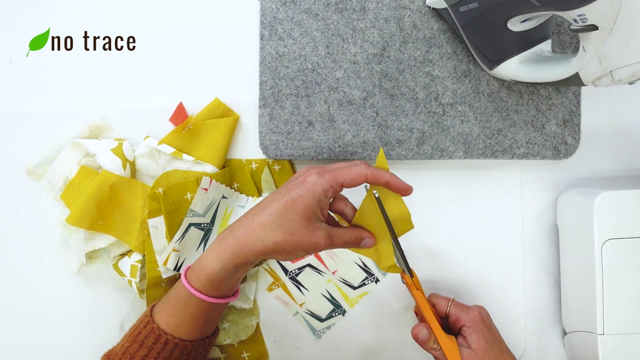 piece to use as the starting point for my little um scrappy drawstring bag. So I'm going to cut this into a smaller triangle and use that as the very beginning. You could start with a triangle, you could start with a square or a five-sided. 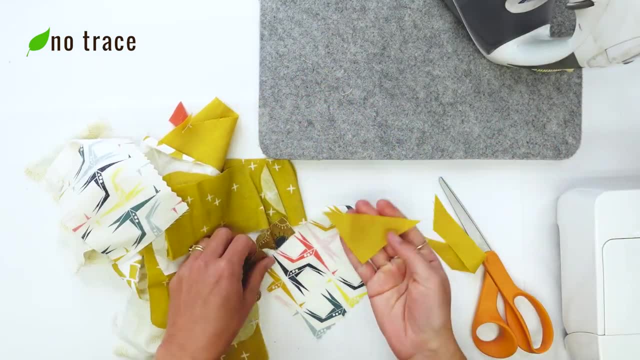 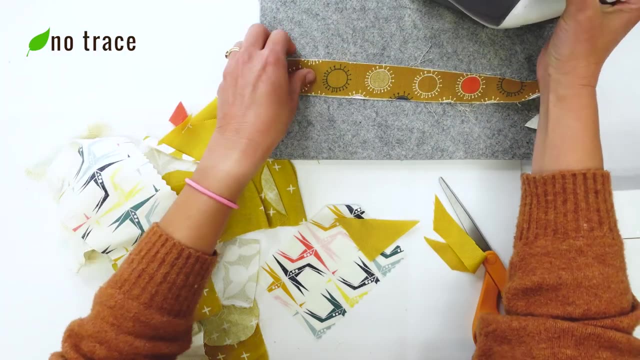 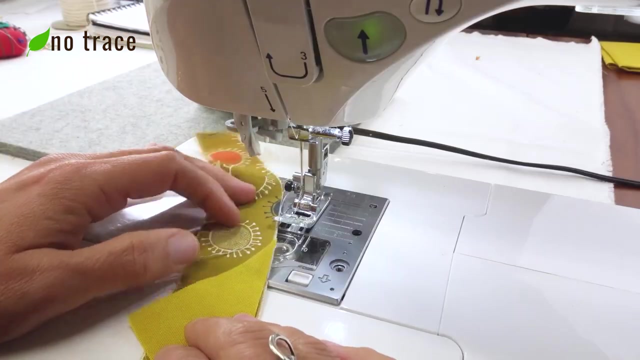 piece of fabric, whatever you want. So I'm starting with this little triangle and then I'm just going to be adding other pieces, pieces, onto it, one side at a time. So I'm going to start with the triangle and this little scrap and sew them with the right sides together. I'm going to use a quarter of an inch seam allowance. 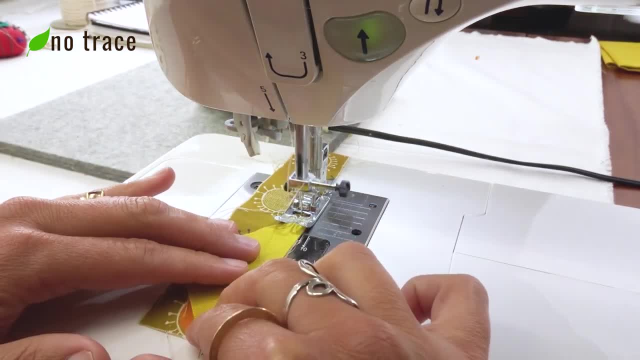 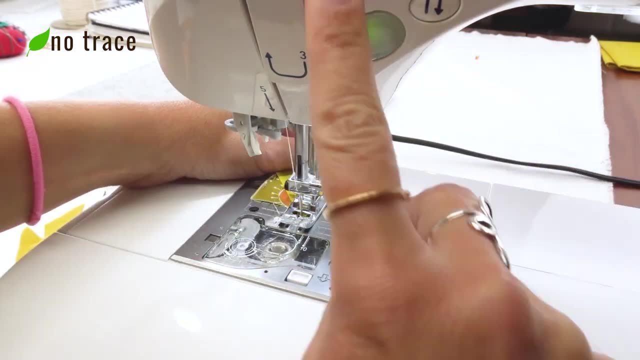 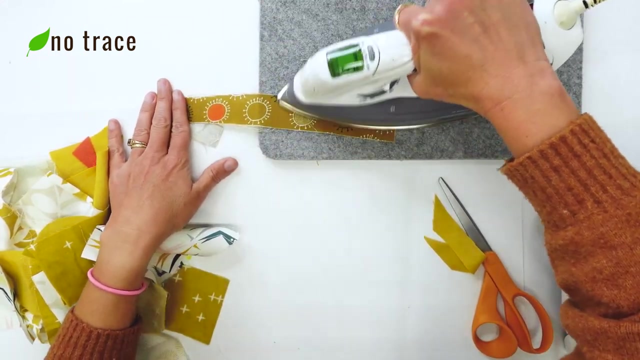 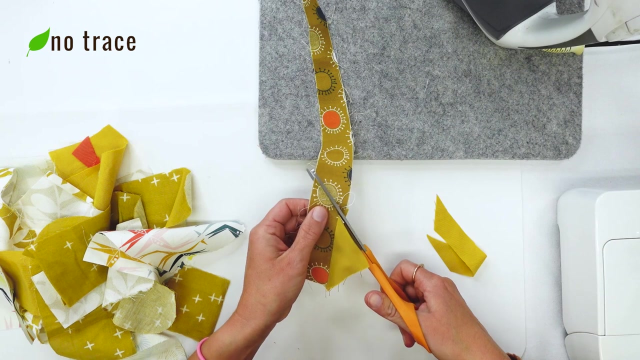 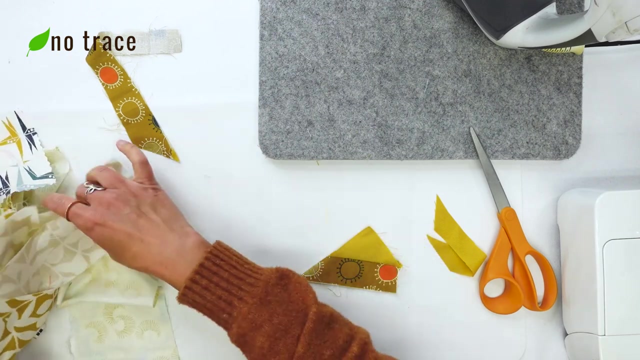 and I'm going to make sure to backstitch at the beginning and the end of my stitches. Once these two are attached, I am going to press them with the iron and then I'm going to cut so that I have another nice straight line to attach to. So now I'll get a second piece, something not too huge, and 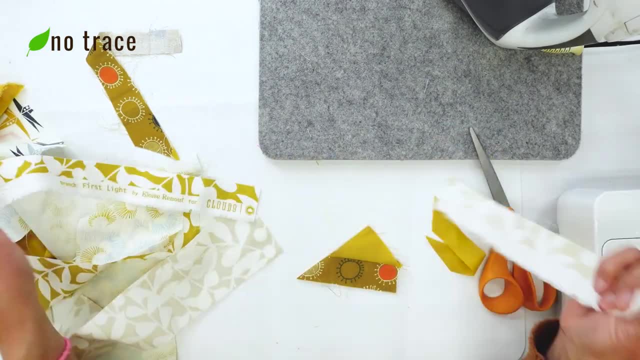 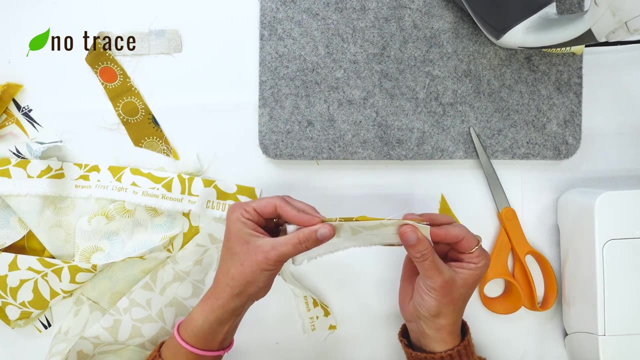 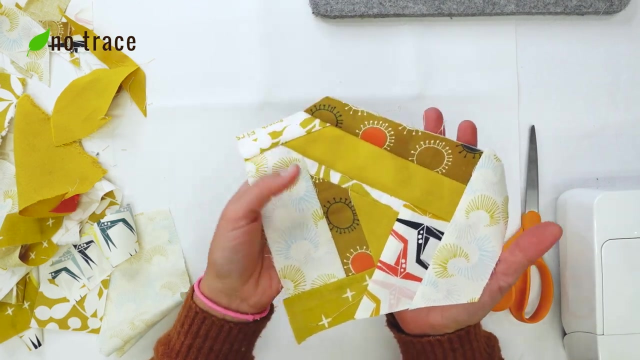 how about this piece? and I'll attach it to This side in the same way. I'm just going to keep attaching pieces of fabric and straightening them out after they're sewn together. Once I have a decent size piece of patched work fabric, I'm 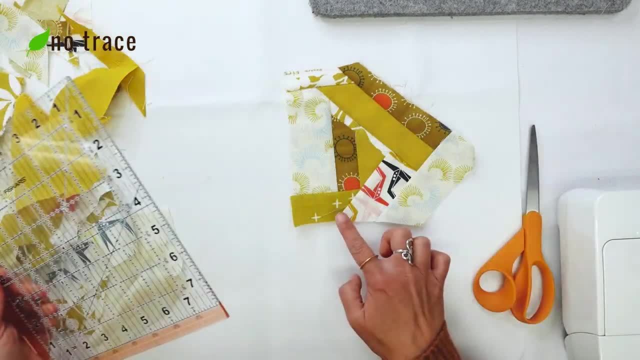 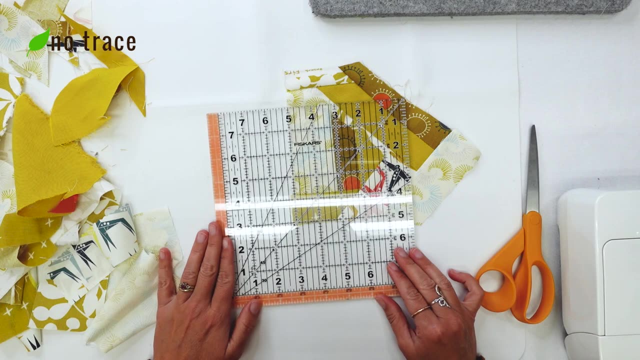 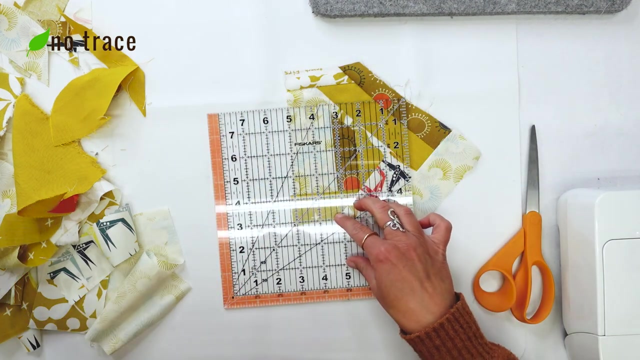 going to get a ruler and I'm going to find a five inch by five inch square in my piece- and hopefully it is big enough and it is. So I'm finding a five by five inch square and I'm going to put it on top of my fabric and I'm just going to mark it out first on two sides. 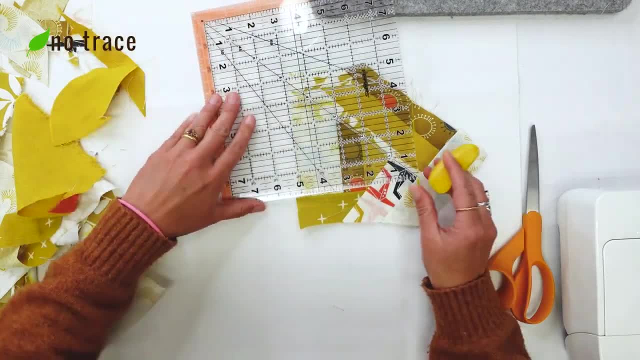 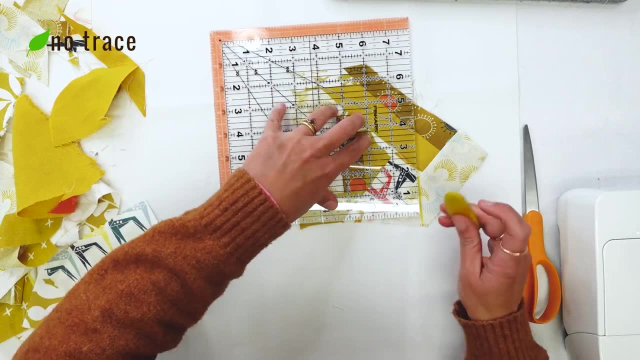 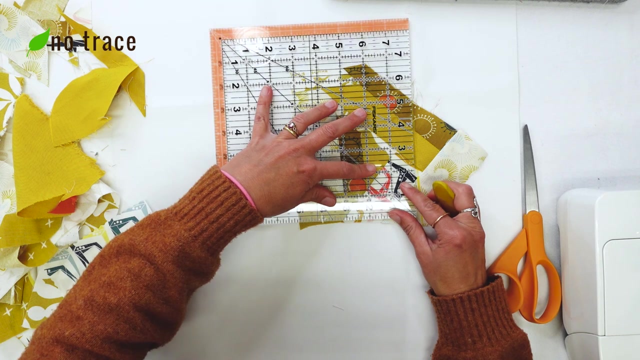 then I will flip my ruler over and mark it out on the other two sides to make sure I have nice straight edges. And if you don't have one of these rulers, you could definitely just use measuring tape and just take your time and mark out a. 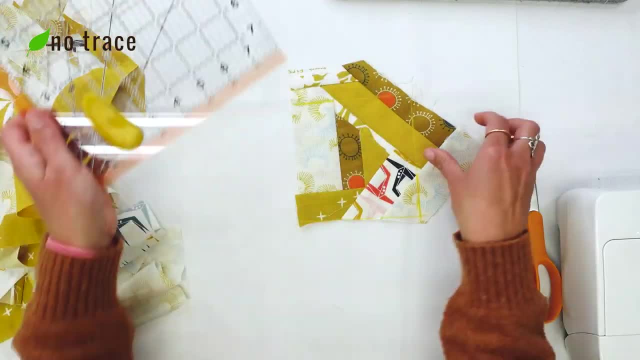 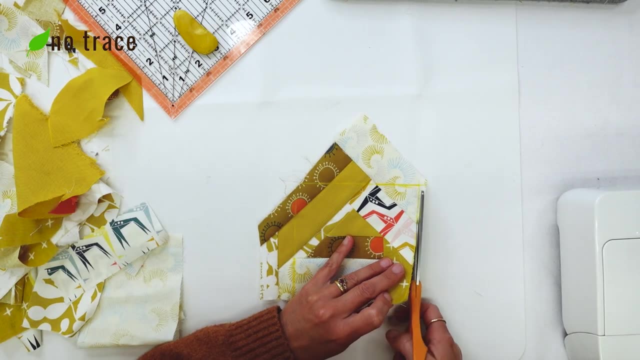 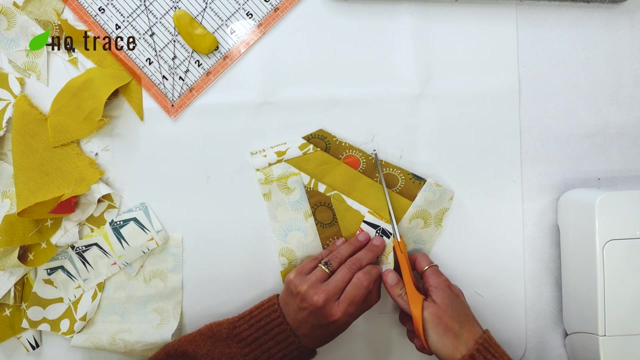 five inches by five inches with your measuring tape. Okay, so I've drawn a square and I'm going to go ahead and cut that out of my patchwork panel here, and once this is cut out, I'm going to go through those same steps and I'm going to make a second patchwork panel that is also. 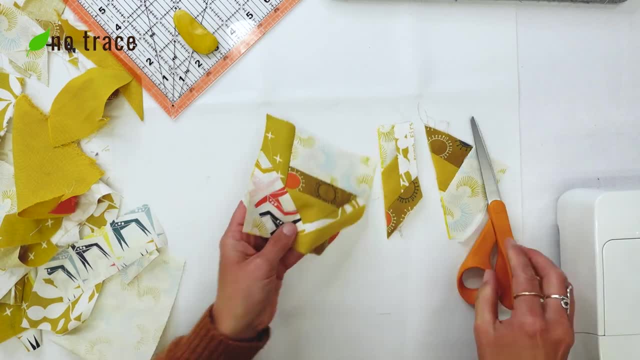 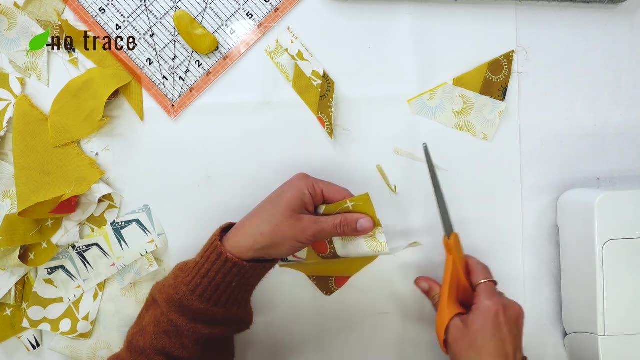 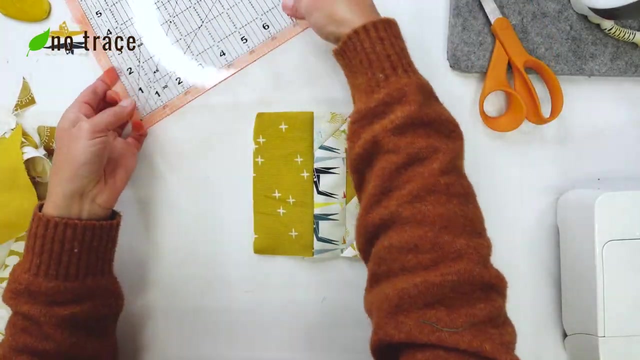 five inches by five inches, and I might use some of these little pieces of fabric. So I'm going to go ahead and set this aside and then start this process with more scraps of fabric. So I've made another patchwork panel here for my little drawstring bag and I'm going 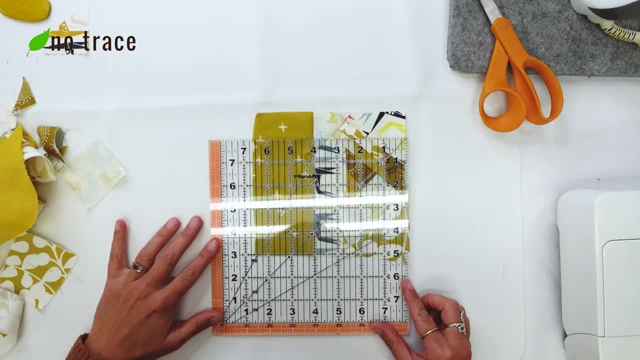 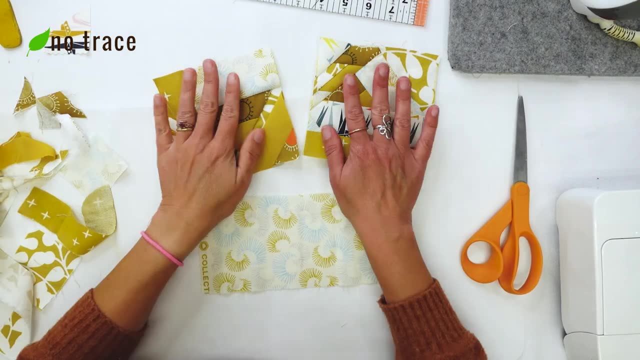 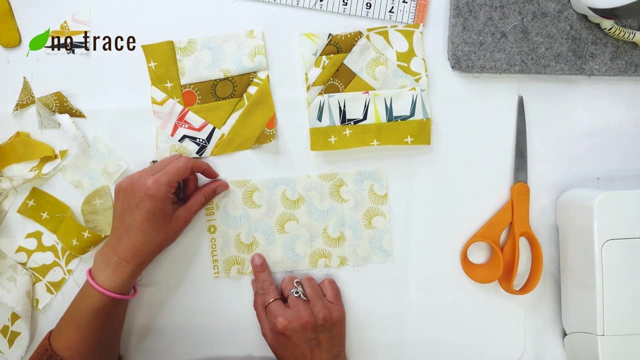 to go ahead and draw another five by five inch square and cut it out with my scissors. Once my two panels for the outside of my bag are done, I'm going to cut out two pieces of fabric that are five inches by two inches, and these are going to become the casing for the. 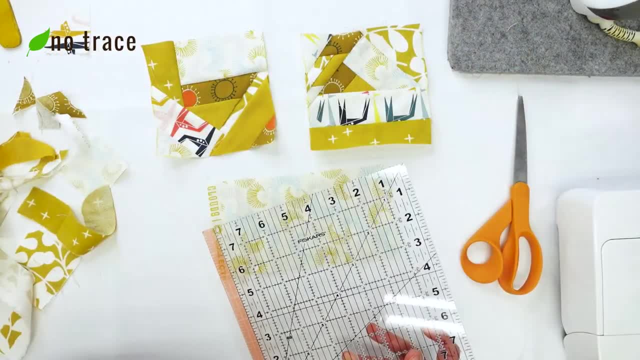 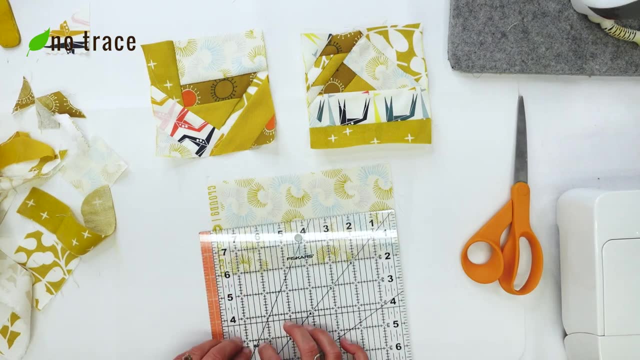 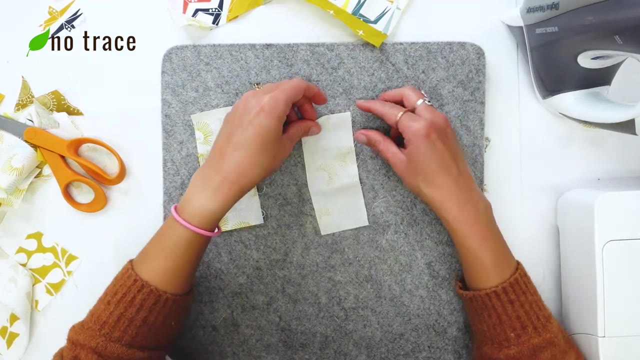 drawstring for the cord to run through. So again, I'm going to get my ruler and I'm just going to cut out a five by two inch rectangle from some more scraps. Once my two rectangles are cut out, I'm going to fold over the short ends about a quarter of an inch, maybe a little bit more. 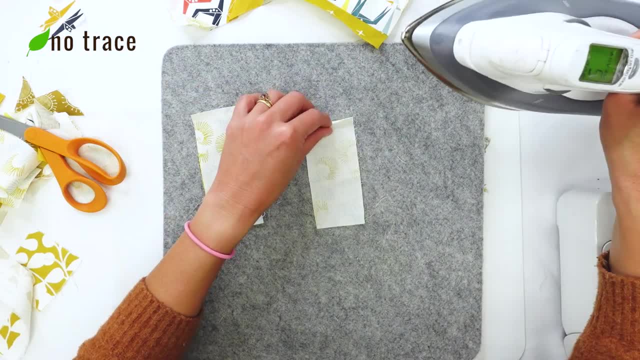 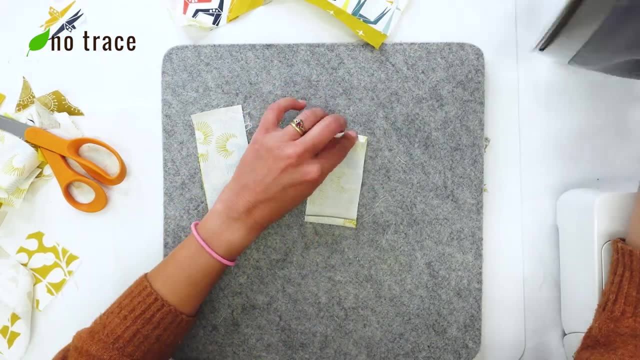 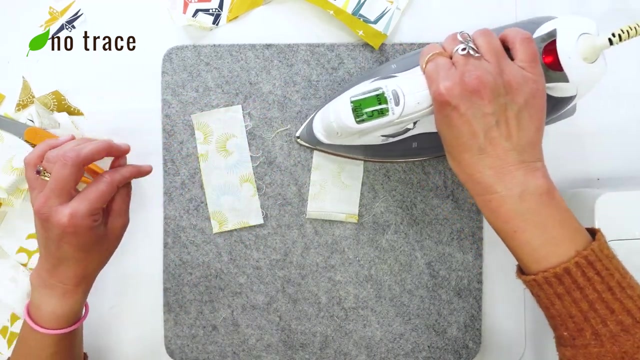 than a quarter of an inch and press it, And then fold it over a second time and press it, and then I'm going to do the same thing on the other short end. So fold it about a quarter of an inch, press, fold and press and I'm going to repeat that. 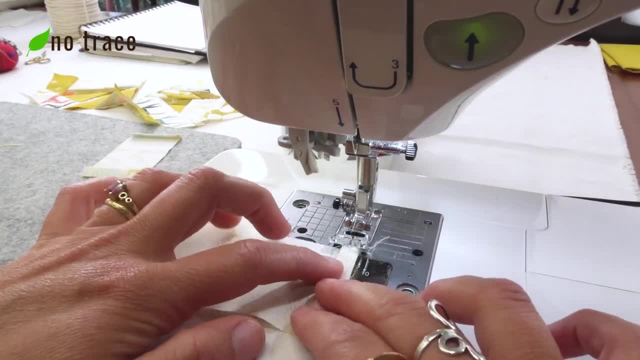 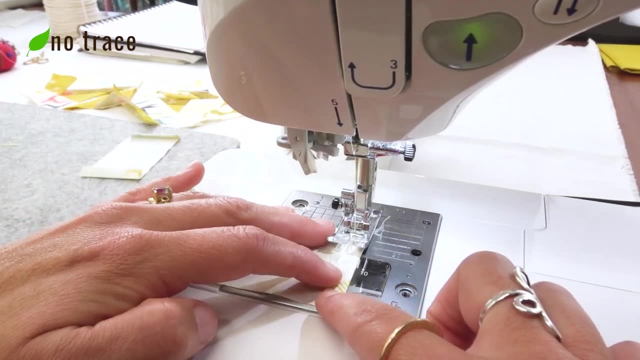 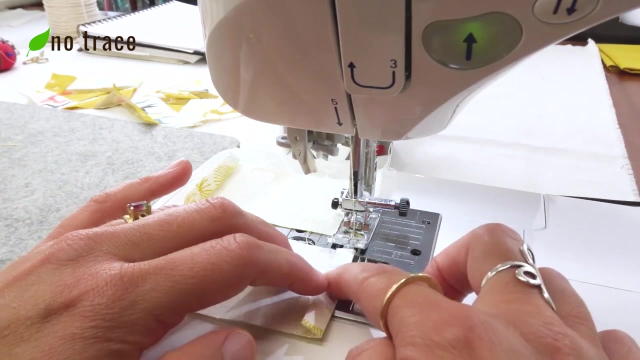 with this little guy And at the machine I'm going to stitch right along this folded edge about with about an eighth of an inch seam allowance away from that folded edge, And I'm going to do that for all four of my little folded over edges. 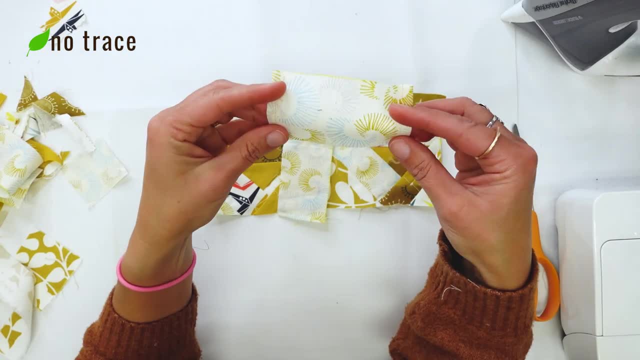 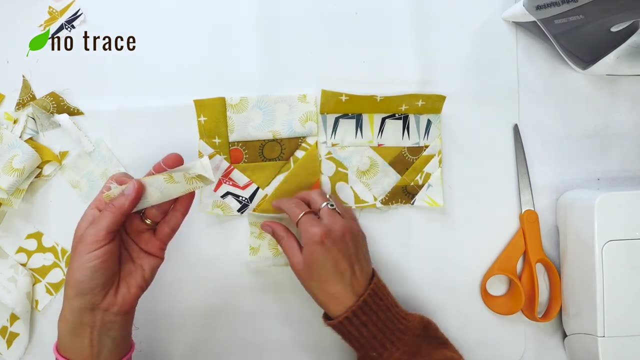 Once I've sewn those edges in place, I'm going to fold the casings in half and then I'm going to be pinning them onto my outside panels. and you're going to want to decide: what do you want the top and bottom to be of your little box? 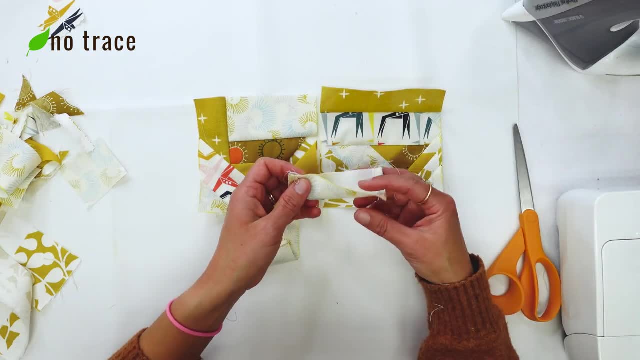 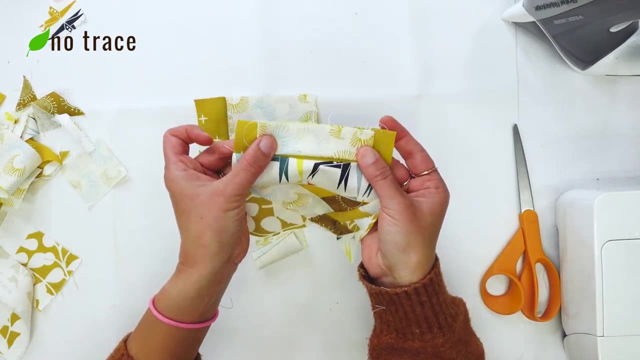 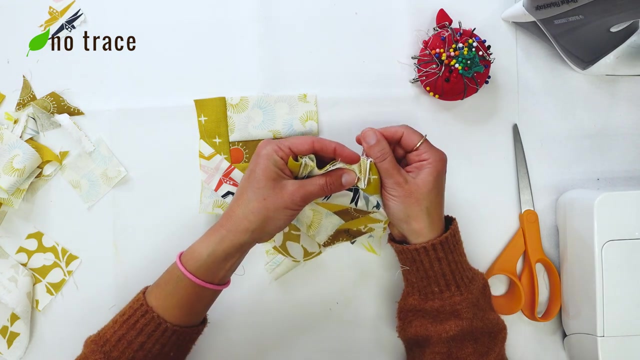 So I'm going to let this, these two edges, be the top edges. Obviously, it's pretty arbitrary because these are little scrappy panels and I'm just sort of eyeballing that I want this more or less centered at the top edge of my outside panel. I'm going to go ahead and put a couple pins there. 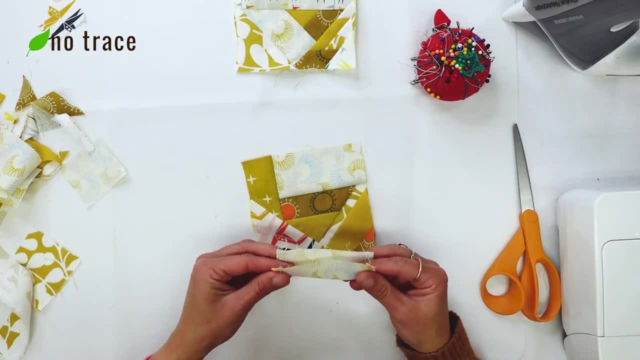 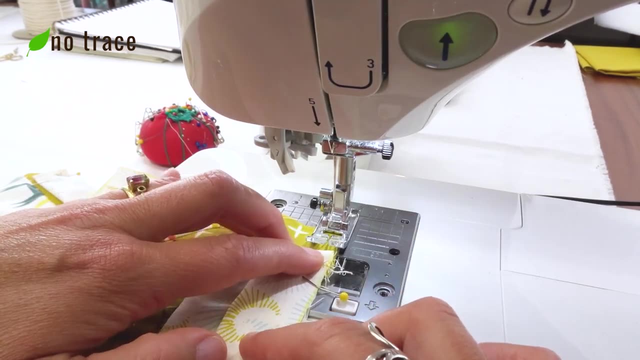 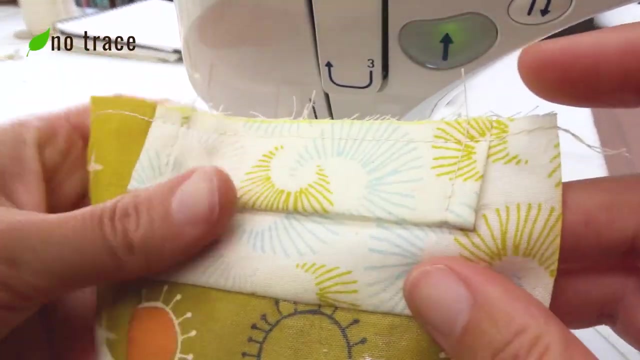 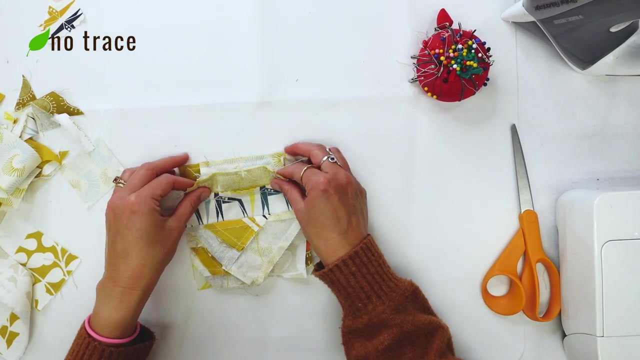 and I'm going to do the same thing on this panel, And once the casing is pinned onto my fabric, I'm going to sew with an eighth of an inch seam allowance, approximately straight down. My casings are in place on both of my panels, so now I want to place these with the right. 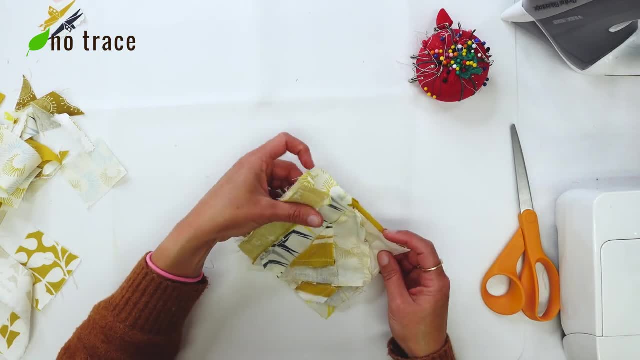 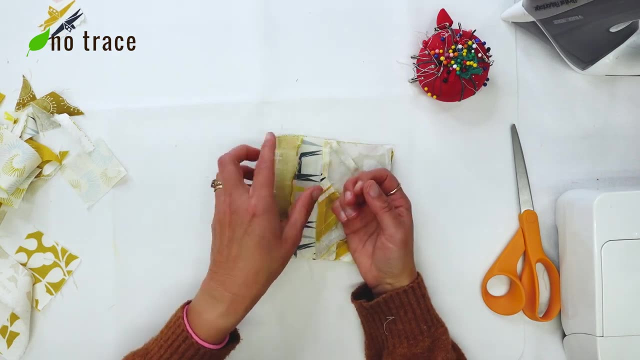 sides together and I'm going to pin them along three sides and then stitch along three sides, leaving this top part of the cases open, And then I'm going to sew them using the other bottom sections. Here I'm going to stitch them on the right side together. Now I'm going to say pretty much all the way around my Consulting. fleet, so that you know the辞arailey effect for everything I just watched. So let me sew with an eighth of an inch seam allowance❢ Adriana's ears im a uphead and I'm going to in place on both of my panels. So now I want to place these with the right sides together and I'm going to pin them among the three sides and then stitch along three sides, leaving this top part with the casing open. 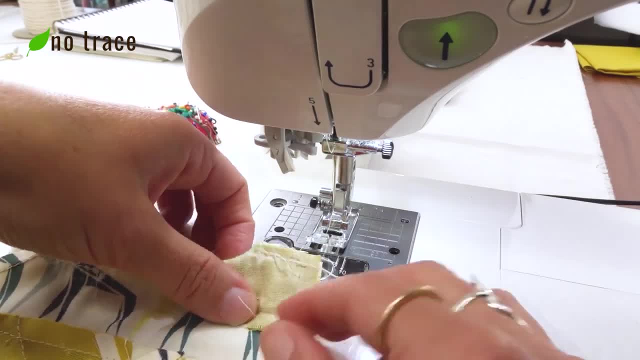 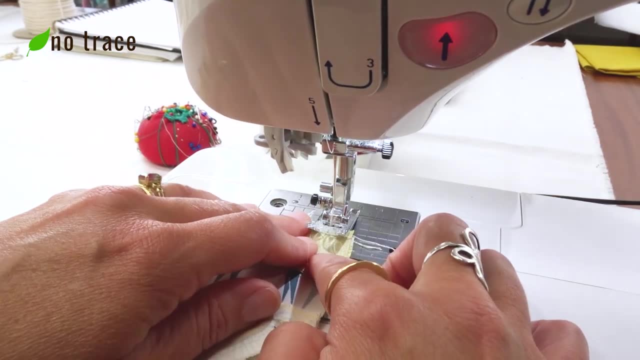 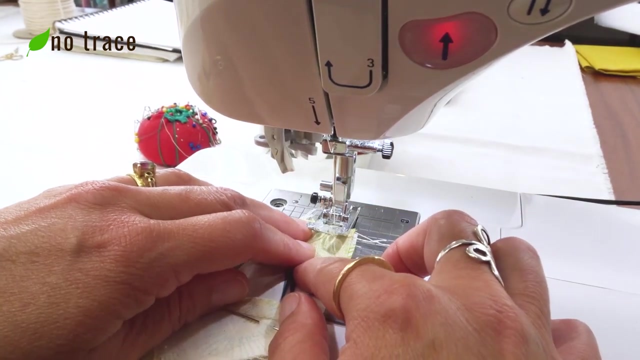 my outer panels with a half inch seam allowance. I want to make sure I don't sew over my casings, so they should be a little bit further than a half inch away. but you could just double check and if you need to move your casings out of the way, you could move your casings out of the way. 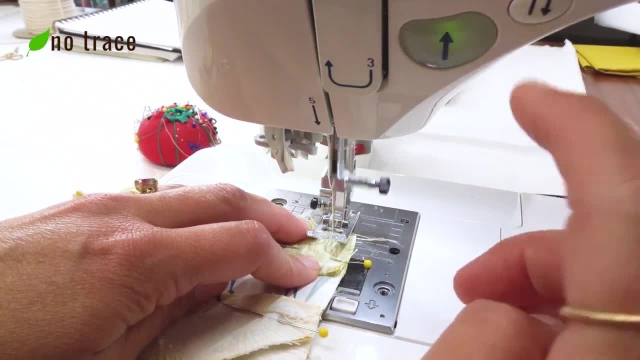 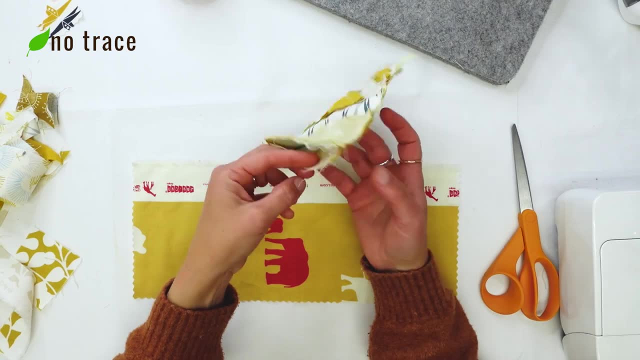 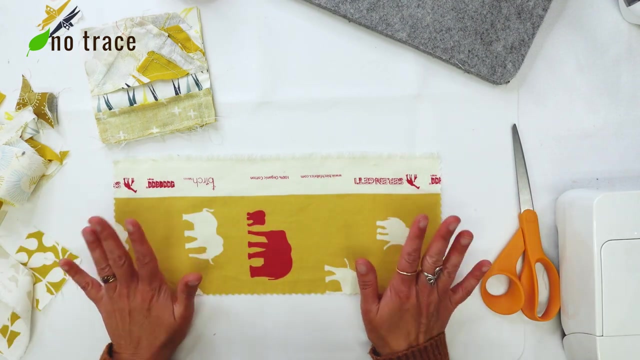 so I'm going to do a back stitch and just go around the three sides. these two are sewn together, so now I need to make the panels for the inside of my bag. this is another great place to use some of your small scraps of fabric. I'm going to be using this. 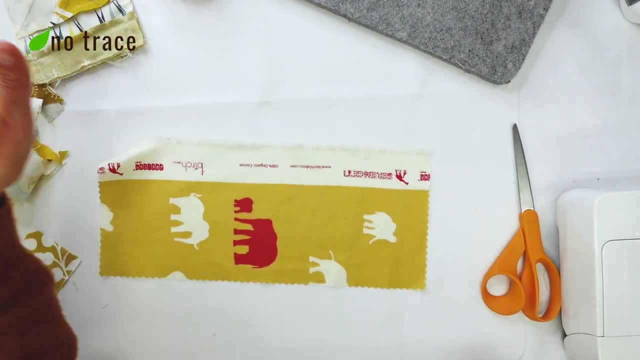 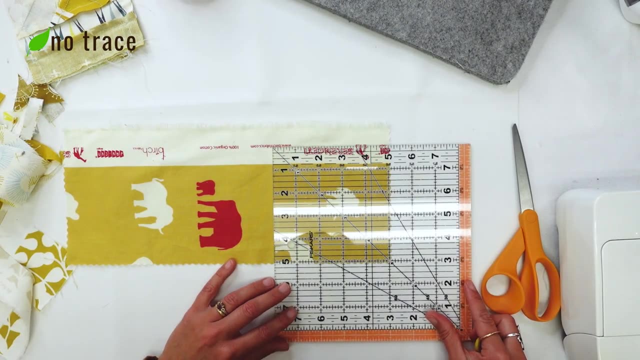 scrap and I'm going to be including this selvedge edge because it's going to be on the inside of the bag. it's not going to be very visible and this is a chance to bust those scraps. so a bit of my selvedge edge is going to show. 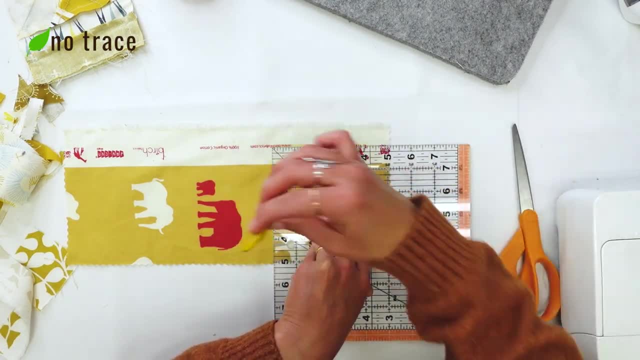 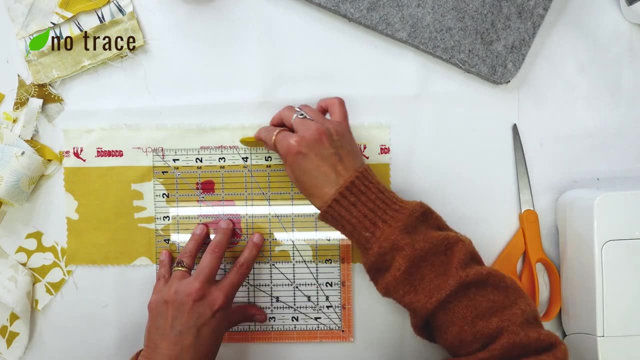 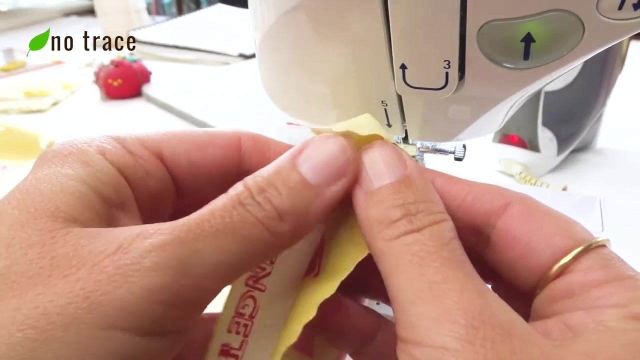 you. that is okay with me. it's going to be on the inside, okay. so I'm just marking out my five by five inch squares, like I did when I was making my outer panels. I'm going to go ahead and cut these now that my two liner pieces are cut out. I've got them right sides together and I'm going to stitch. 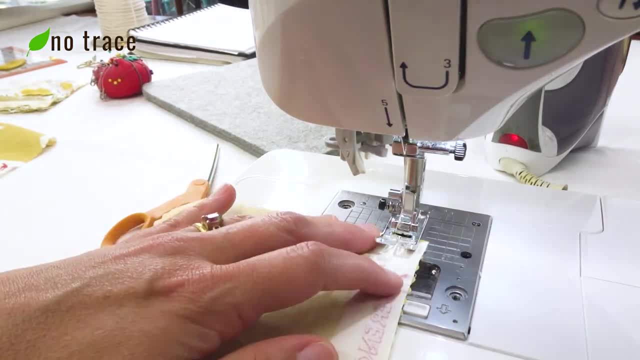 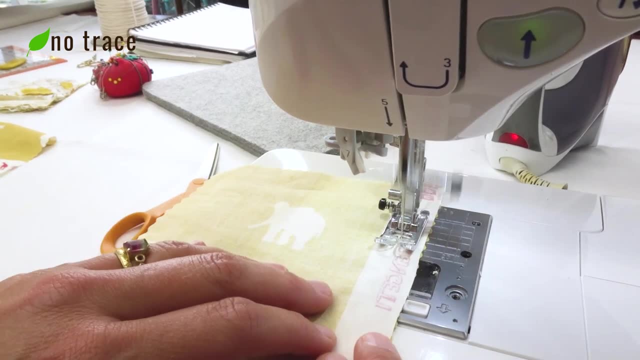 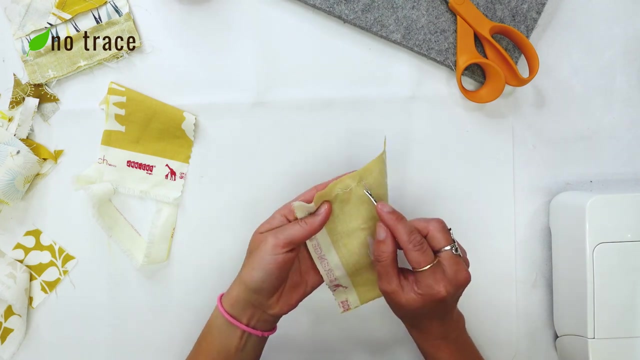 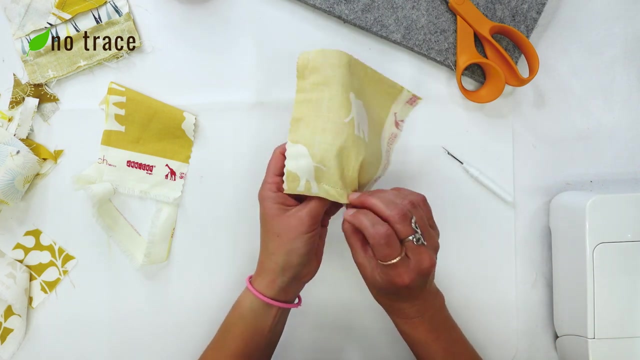 around three sides with a half inch seam allowance, making sure to back stitch at the start and stop them off. sourced gave a nice curve to this 예 and I forgot to leave an opening in my liner fabric, so I'm Gonna just Seam rip about three inches in this bottom seam so that we can turn the whole bag right side out. so you need an opening. 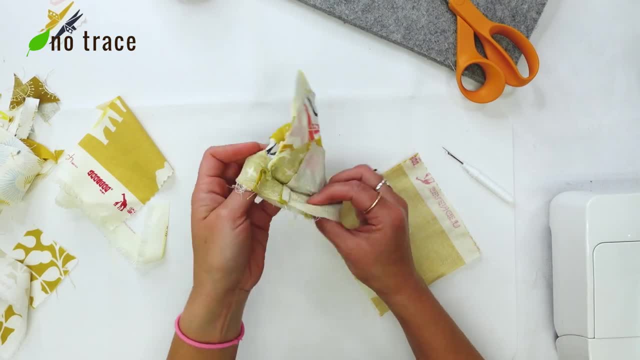 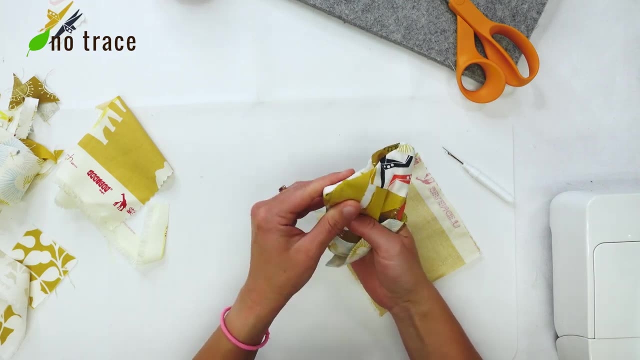 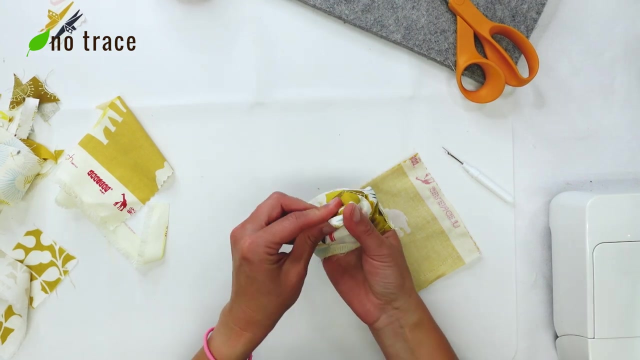 about like that. now I'm going to take my outer panels that are all stitched together, turn it right side out. I'm going to push those Corners out much as i can. you could snip the extra fabric off your corners if you want. i'm just going to push. 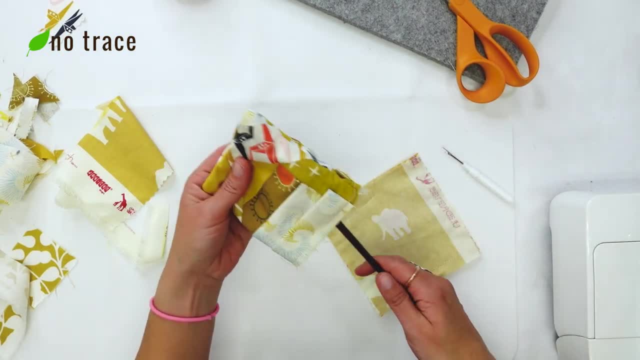 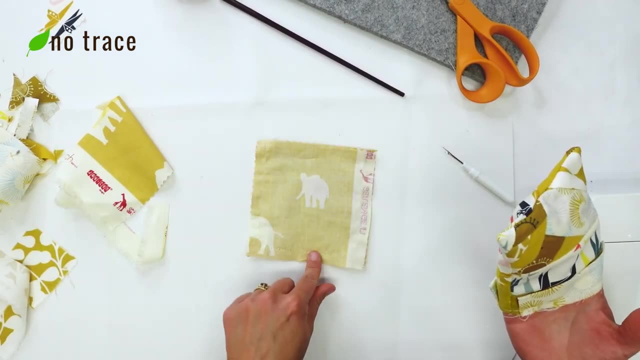 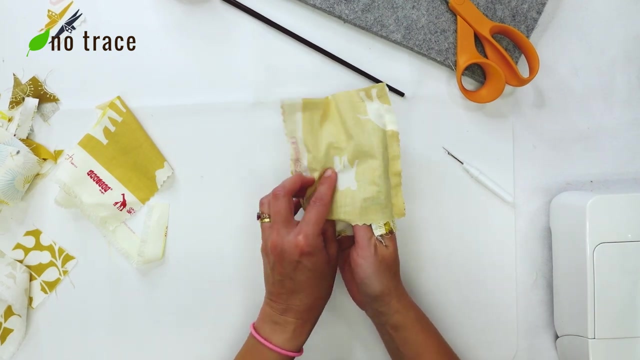 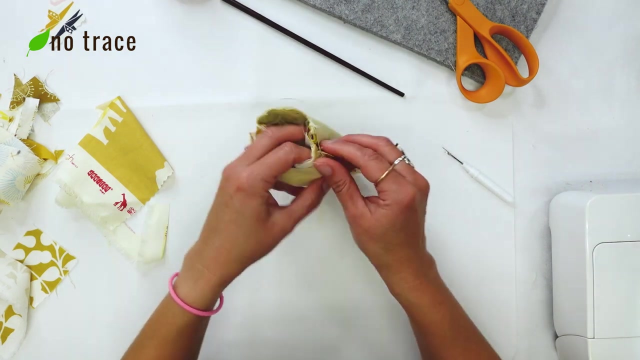 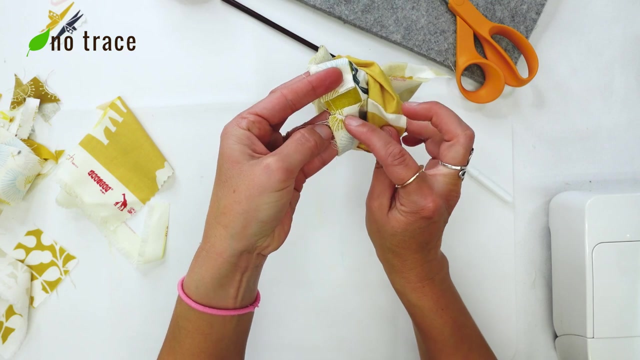 them out with my chopstick, just take a moment. and then i'm going to put this in between my inner layers. just slide it on in there. hopefully it fits nicely. and then i want to line up the side seams. so i want to line up the side seam from my liner fabric with the side seam of my outer fabric. 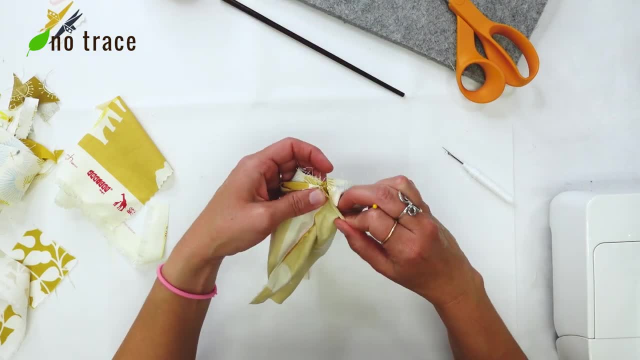 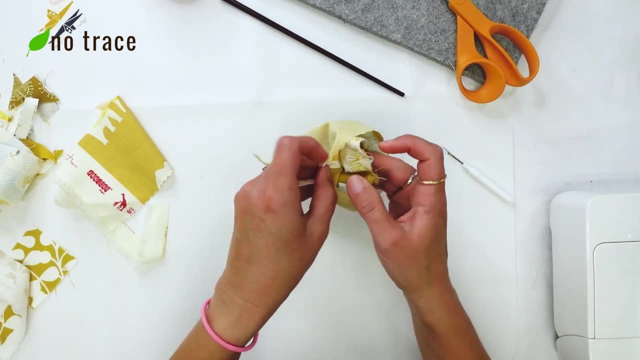 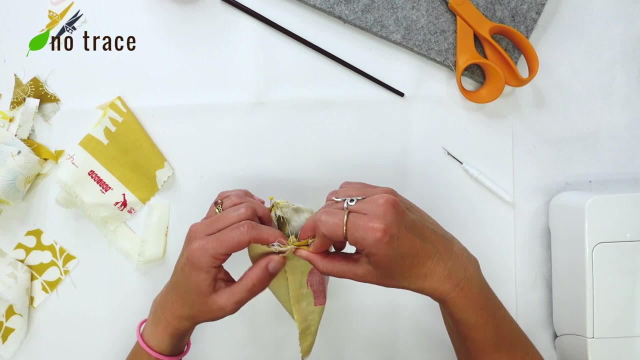 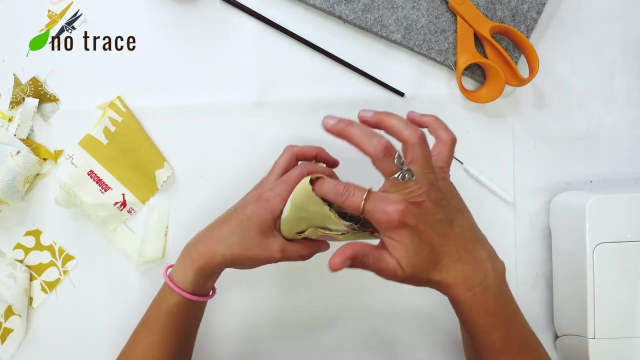 and pin so that they stay together. let's get it pinned in there and then do the same thing on this side. so line up the outer- sorry, the inner- fabric seam with the outer fabric seam nicely, and pin them together, and then we're going to stitch around this edge with a half inch seam allowance, since this is a pretty narrow opening. i'm going to 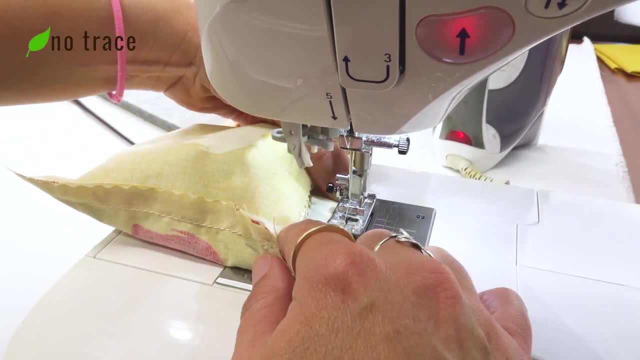 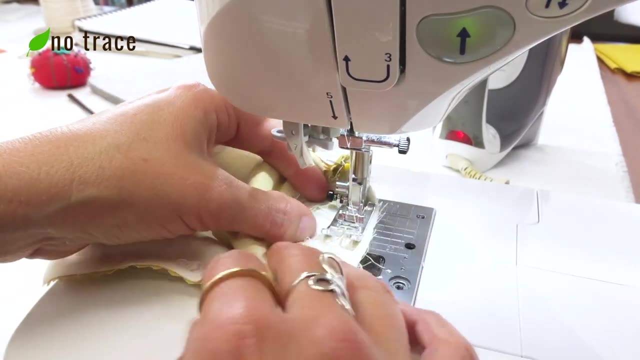 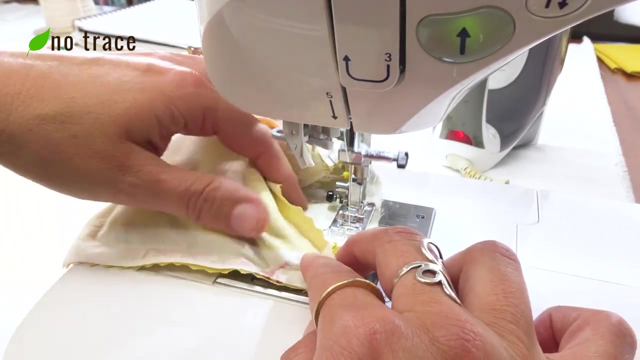 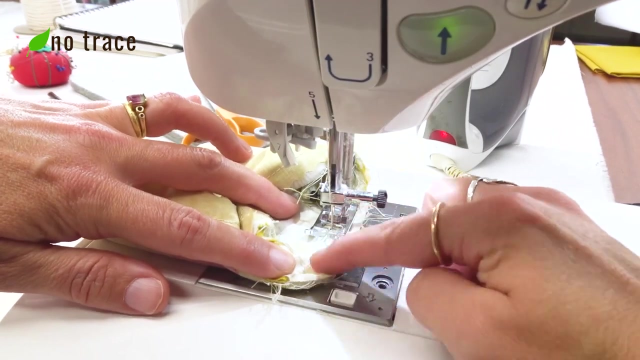 be stitching around the inside here. so i'm going to lift my presser foot and get the bag underneath and and i'm going to be holding one side away from the presser foot and just go all the way around. i'm coming up to where i started sewing and i'm just going to follow this row and try to get. 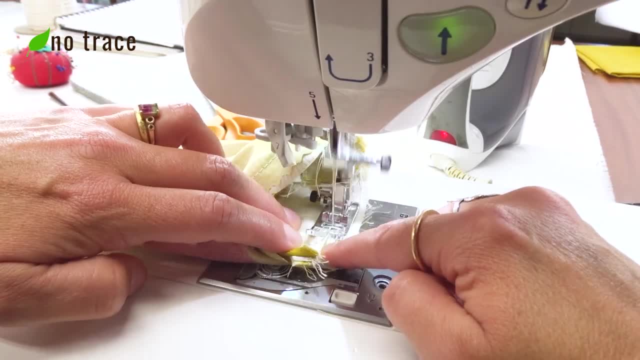 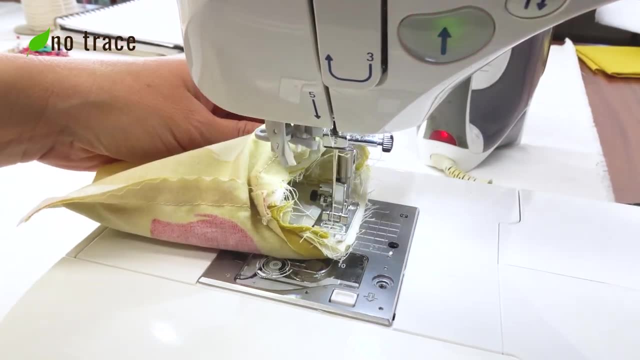 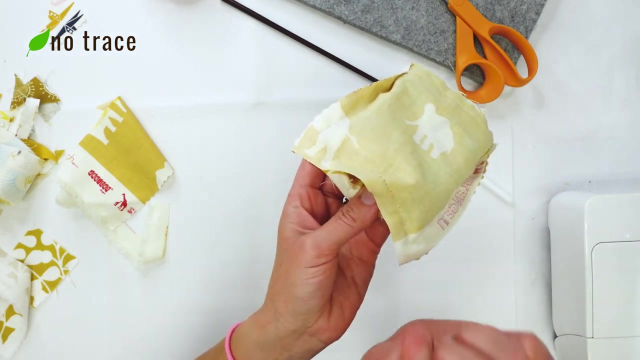 right on top of this original row with a few stitches and then i want to do a back stitch. once this top seam is done, i'm going to use the little opening i left in the bottom of the liner fabric. actually, i didn't leave that opening, i seam ripped that opening. 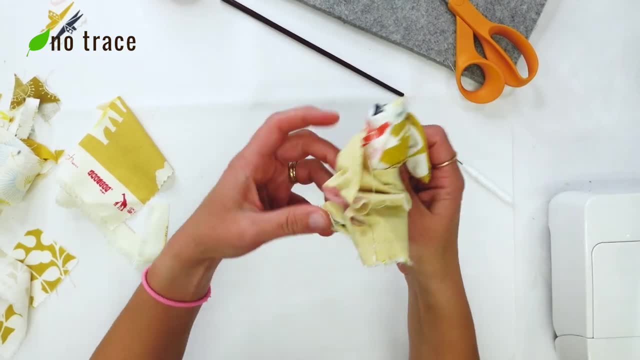 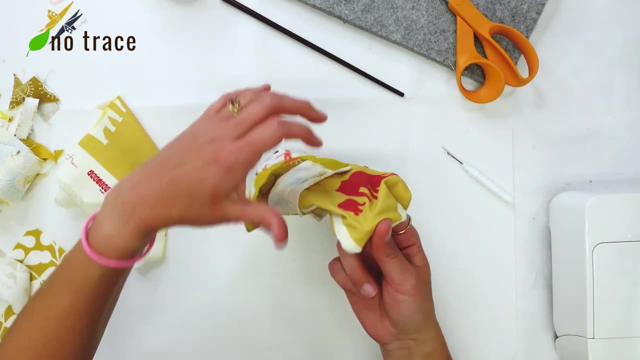 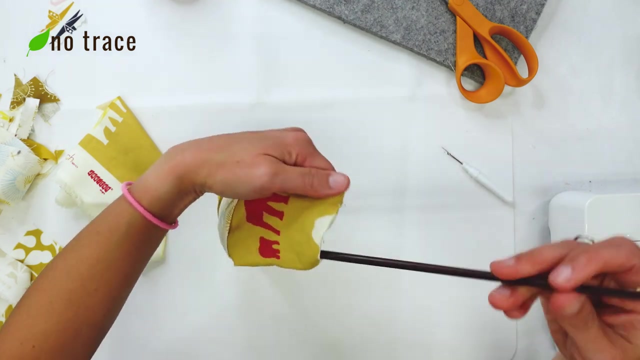 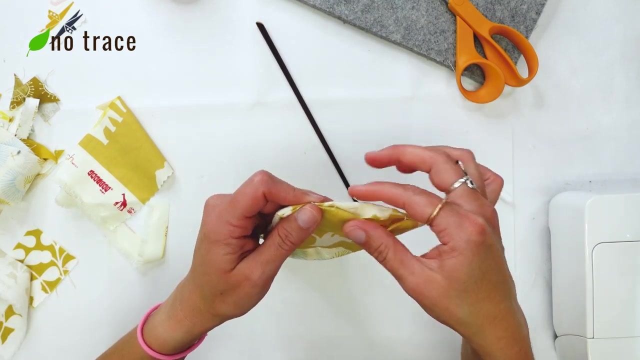 and i'm going to pull the outer panels through the inner panels and i'm going to flip my inner panels right side out and then i'm gonna push out these corners nicely and then I want to finger press the opening and sew it closed with a simple top stitch. 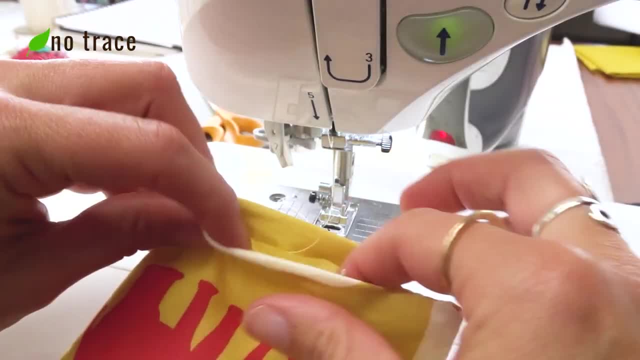 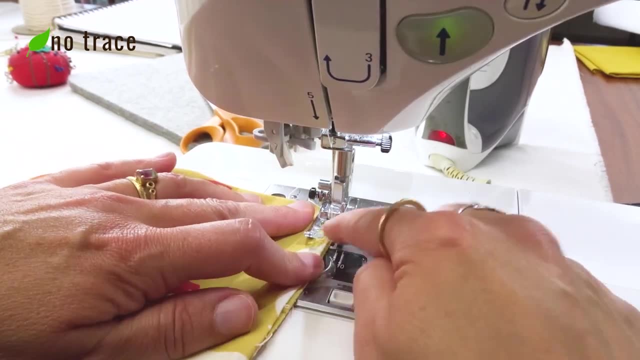 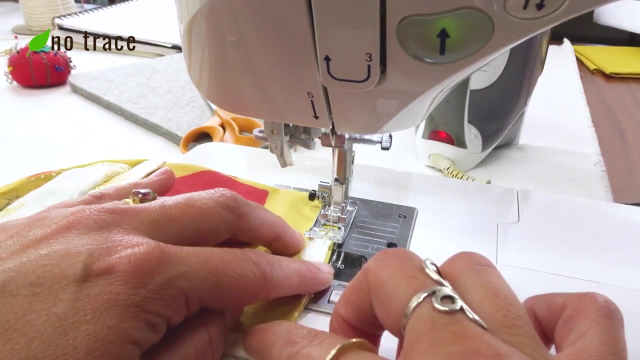 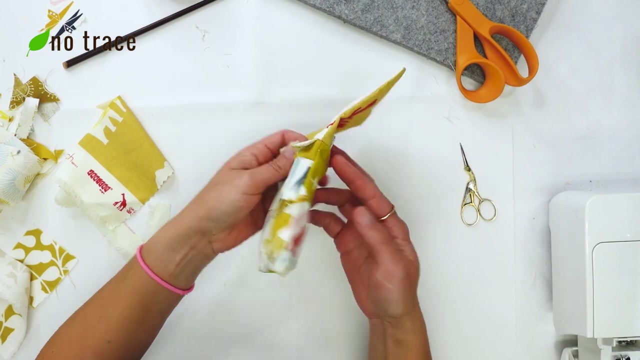 all right, just make sure that the raw edges are folded in nicely with each other, and we're just going to sew straight down, and I am going to do a back stitch at the beginning and the end. I like to take a moment and tidy up all the loose threads. once everything is tidied, all you got to. 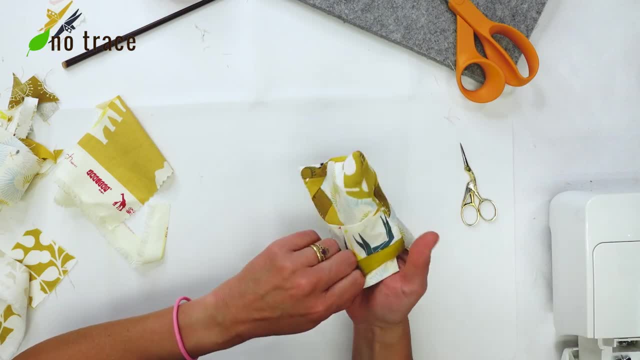 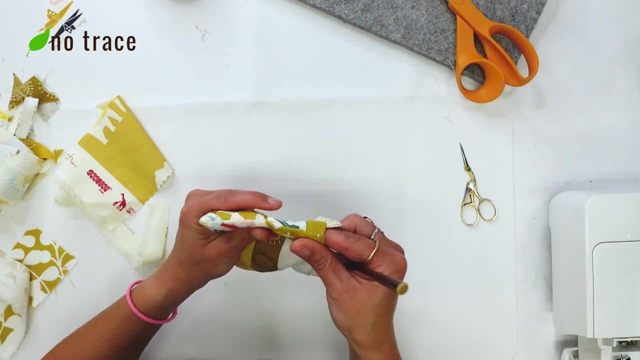 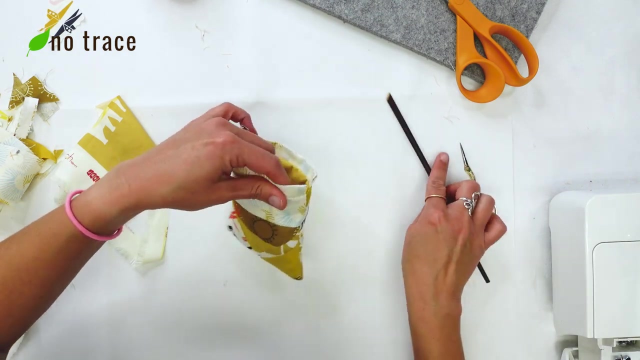 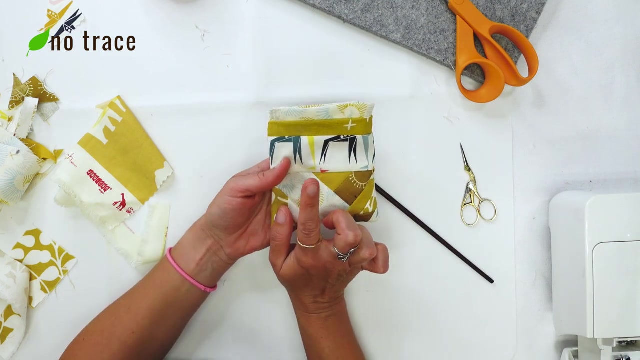 do is push the liner fabric into the outer fabric. this bag is so cute. there's something so fun about making tiny things. I don't know. can you relate- leave a comment below you. if you can relate- to the satisfaction of sewing small things, okay, I want to do one more seam. I'm 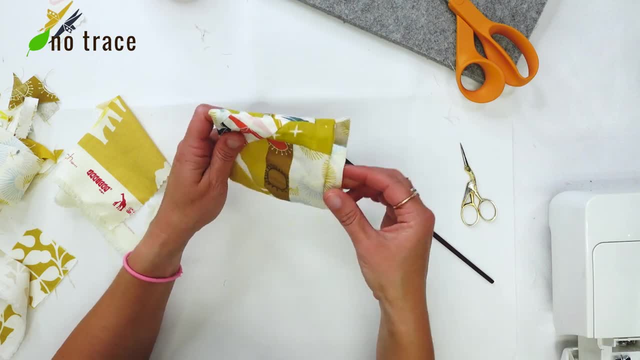 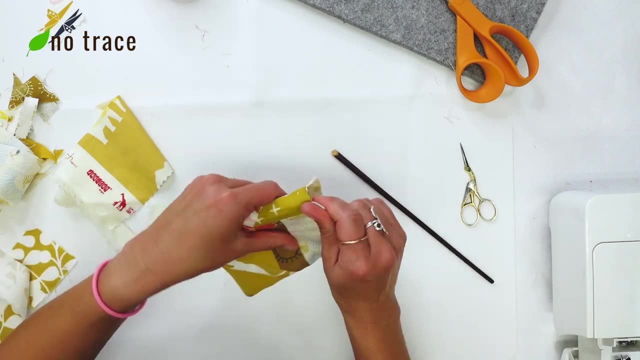 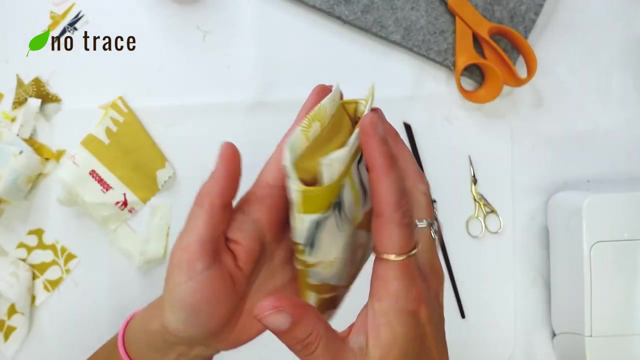 going to do a top stitch around this edge, leaving the casings opening open. just right below the casings I'm going to do one more row of stitches just to give it a little bit more of a polished finished look. so I'll be right back. so I did a little top stitching there just to give it a 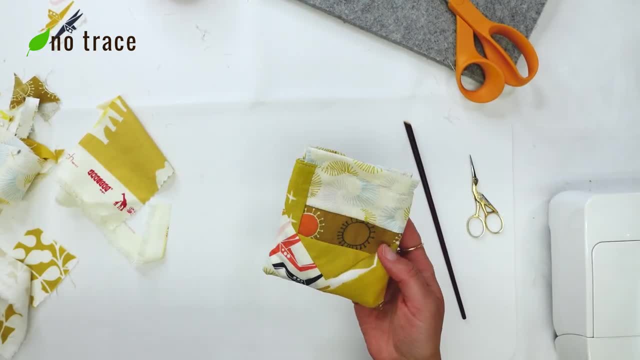 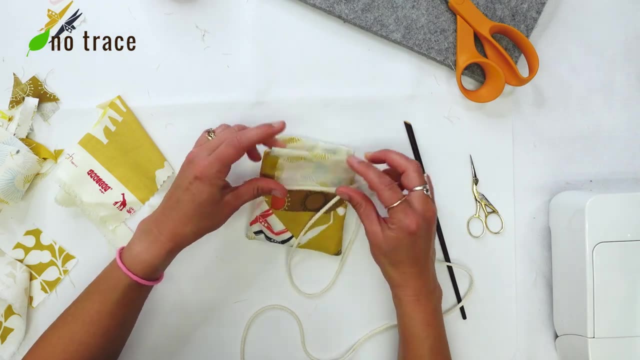 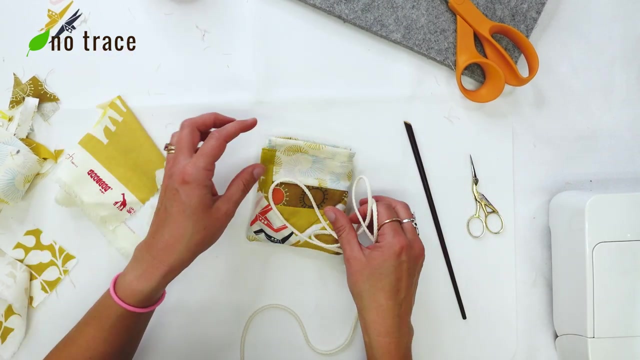 little extra pizazz, and the next thing we're going to do is the last thing we're going to do, which is thread rope through the casing. you could use shoelace for this. this is some organic cotton cording. you could use a ribbon- really, whatever you have on hand, that'll fit in the casing, will. 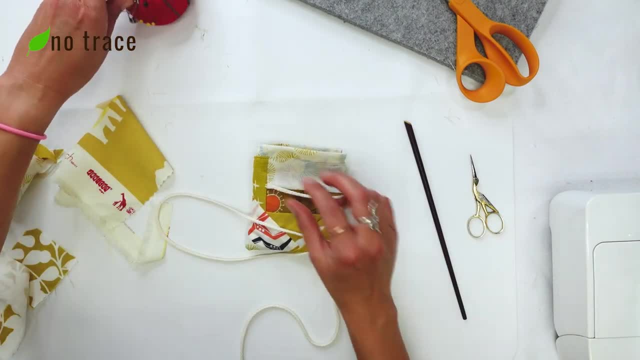 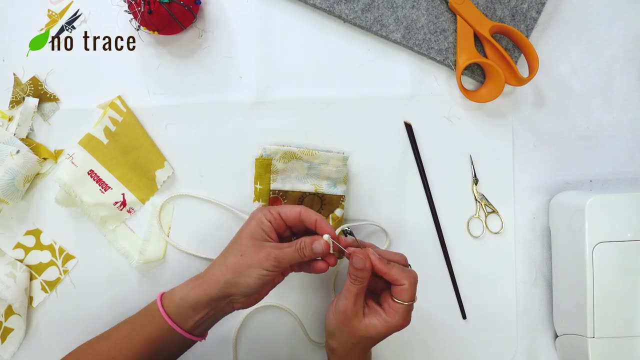 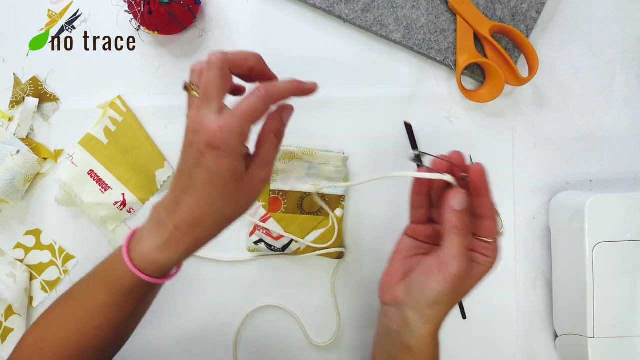 work perfectly and I am going to grab a safety pin. by the way, if you're getting any value out of this video, I would love a thumbs up, so go ahead and subscribe to my channel and I'll see you in the next video and do that. all right, I'm going to safety pin the cord onto the pin and slip it in. actually, this: